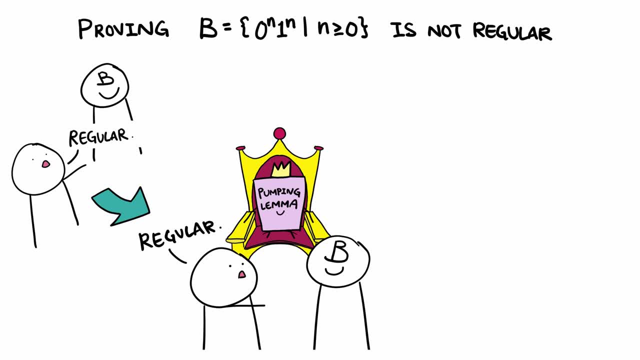 it to the all-knowing pumping lemma. that gives us back the pumping length p, which, if you recall, if a language is regular, then for all strings in the language that has a length of at least p, there will be a section of the string that can be pumped and still be in the language. 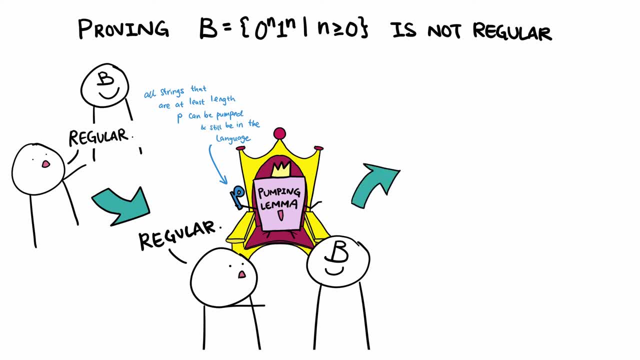 Now given p. this next step is where we show that the language is actually not regular. We have to find a string that is at least length p that breaks the pumping lemma. So, for our example, 0 to the n, 1 to the n. this string, 0 to the n1, limited to 5, because roots belongs to a. 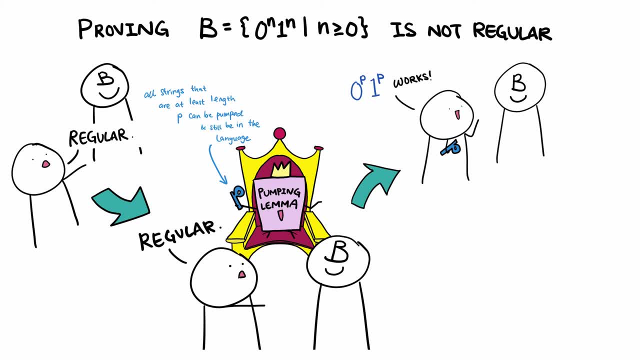 0 to the p. 1 to the p is indeed at least as long as p, but cannot in fact be pumped. We will use this string to contradict our initial assumption that the language satisfies the pumping lemma, And since we had claimed that the language is regular according to the pumping lemma, 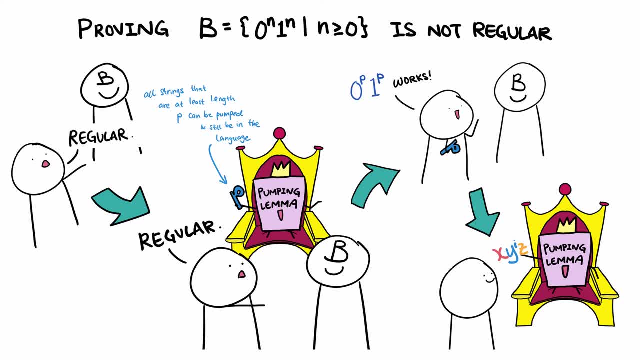 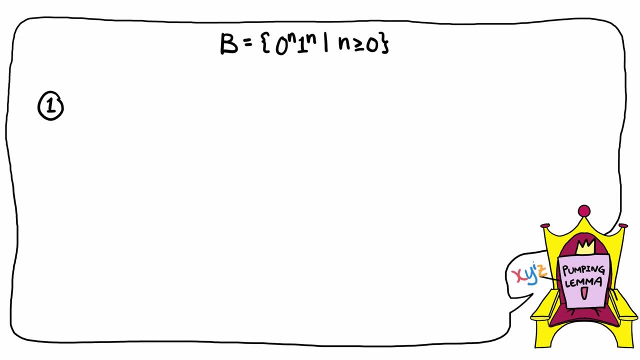 the string can be split into three different components: the part before pumping, the part being pumped and the part after pumping. And this is where we see things go wrong and the contradiction kicks in. We can argue that there are three cases for how the pumping lemma could have chosen y. 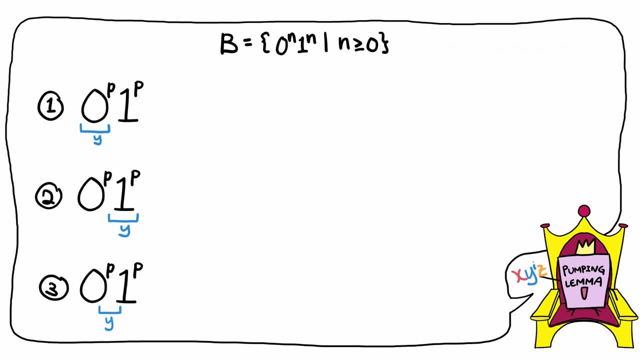 It could have chosen all 0s, all 1s or a combination of 0s and 1s as the pumping string. If the pumping string consisted of all 0s, then we will end up with a string that has: 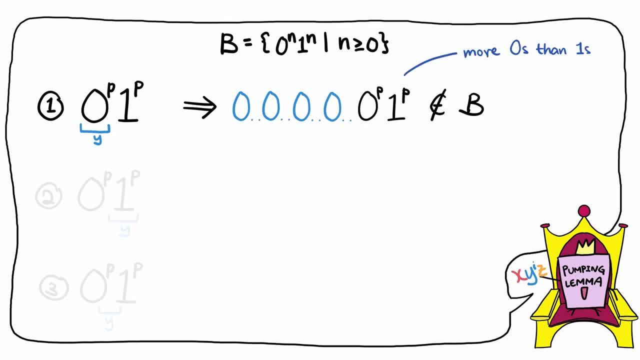 more 0s than 1s, Which doesn't belong in the language. Similarly, if the pumping string consisted of all 1s, then we will end up with a string that has more 1s than 0s, which also does not belong in the language. 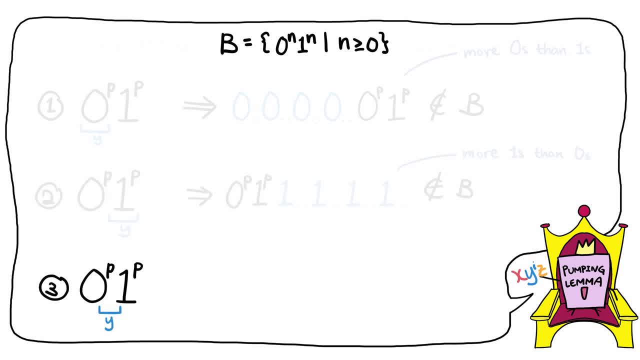 And if the pumping string y was somewhere in the middle where it consisted of both 0s and 1s, then we may end up with a string with a different sequence which also does not belong in the language. Therefore, this string is not a pumping string.